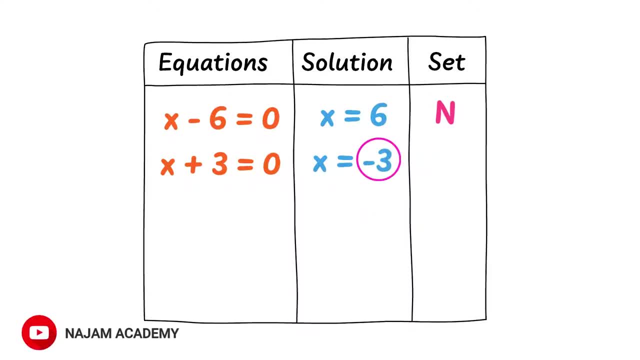 equal to minus 3.. Minus 3 is a negative integer and belongs to a set of natural numbers. We know that its solution is: x is equal to minus 3.. Minus 3 is a negative integer and belongs to a set of natural numbers, So the solution of this equation lies in the set. 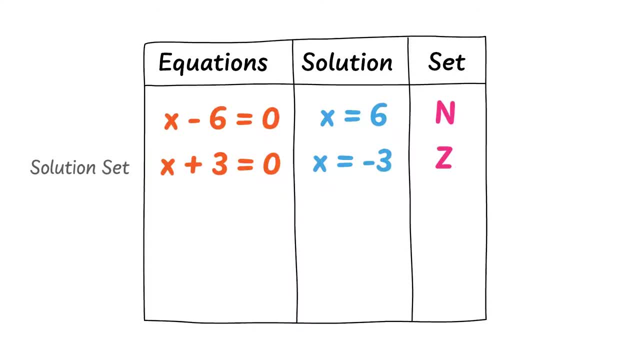 of integers or real number. Thirdly, consider: 3x minus 2 is equal to 0. We know that the solution of this equation is: x is equal to 2 divided by 3.. 2 divided by 3 is a rational number, or it belongs. 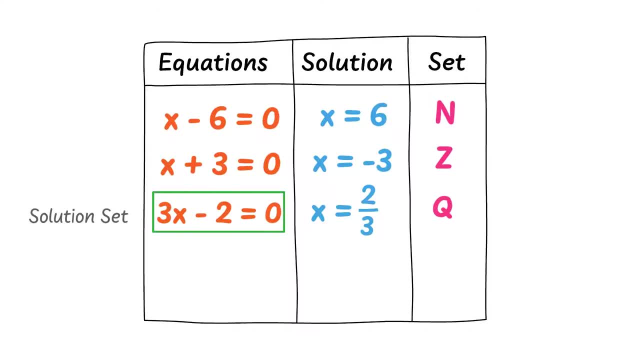 to a set of q. The solution of this equation lies in the set of rational number or real number. Fourthly, consider: x squared minus 3 is equal to 0. We know that its solution is: x is equal to plus minus square root of 3.. What about plus root 3 and negative root 3? Well, plus root 3 and. 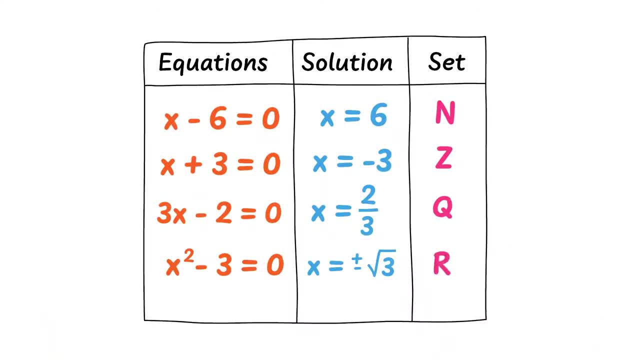 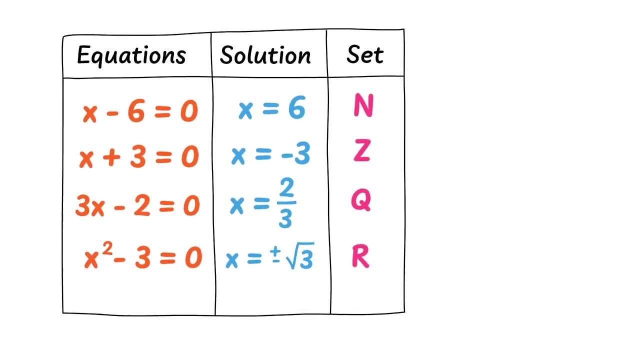 negative root 3 are irrational numbers, So the solution of this equation lies in the set of irrational numbers or real numbers. Finally, consider: x squared minus 3 is equal to 0.. We know that its solution lies in the set of irrational numbers or real numbers, So let me solve it. 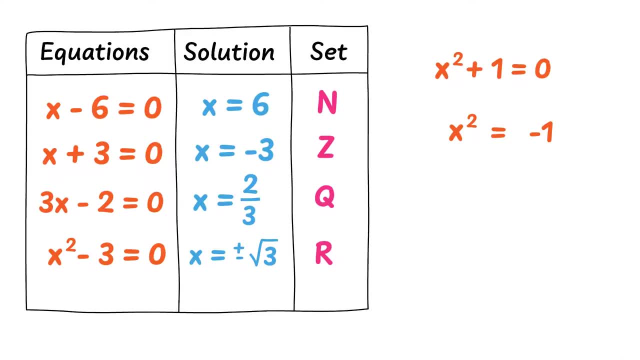 We can write it as: x squared is equal to minus 1.. Taking square root on both sides, we get: x is equal to plus square root negative 1, or x is equal to negative square root negative 1.. Well, we know that root negative is neither a rational number nor a rational number, and 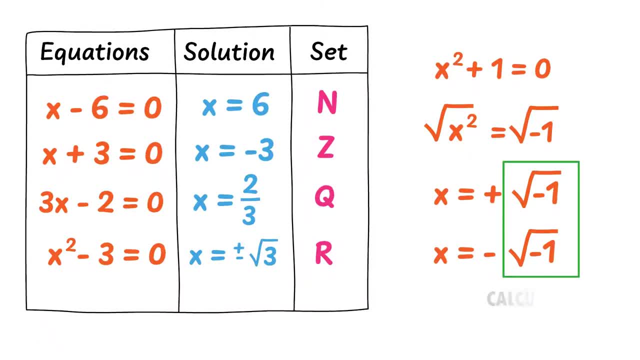 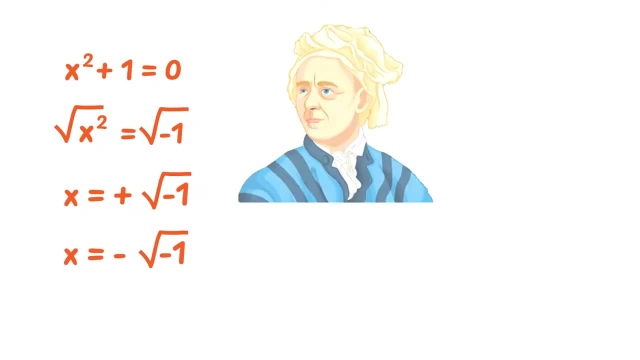 can't find the value of root negative 1 using calculator. that's why in the school we used to say that there is no solution for this equation, or this equation has no solution. but now you are going to learn its solution. it was Euler who give a symbol, I, to the square root of negative 1 and called it unit. 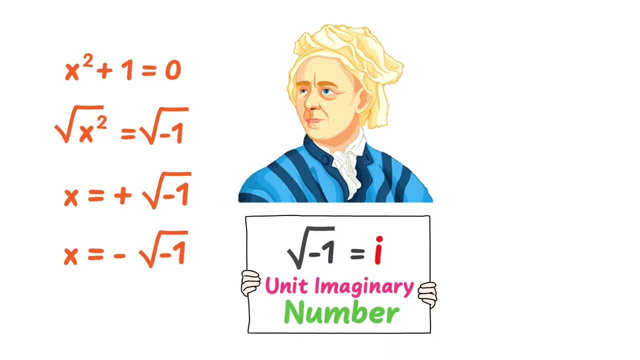 imaginary number because we can only imagine square root of negative 1 and it is thought to be impossible this. whenever you see square root of negative 1, remember that it is always equal to i, a unit imaginary number. now we can solve this equation easily by the help of unit imaginary number. like x squared is equal.